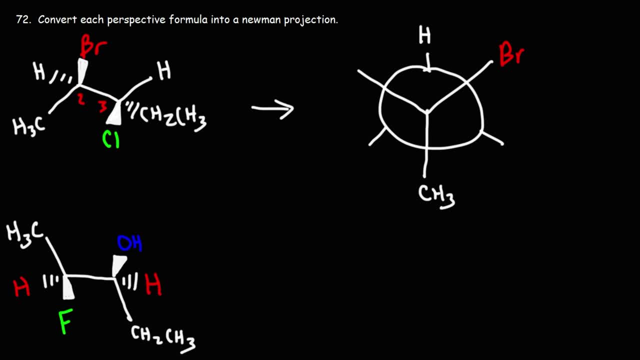 So here's bromine in the upper right side, Because it's on the wedge, it's coming out of the page. And here's hydrogen in the upper left side. It's on the dash, It's going into the page. Now, moving on to carbon 3.. 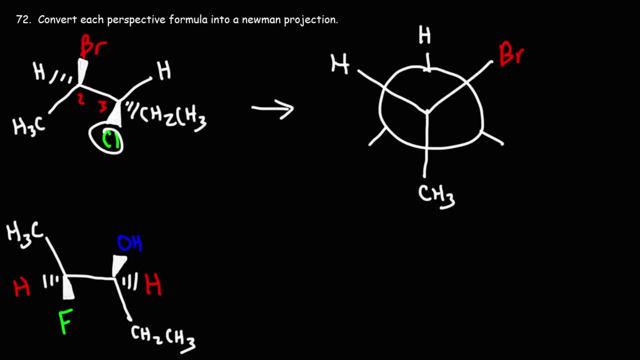 The chlorine atom is on the wedge, coming out of the page, So we're going to put that on the right side. The same with the bromine atom. The ethyl group is on the dash. It's going into the page, So it's going to be on the same side as hydrogen. 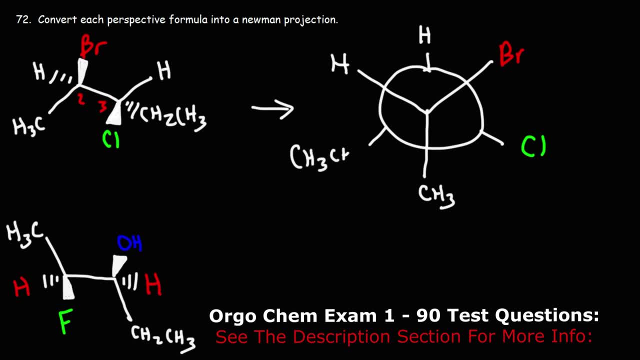 That is on the left side but attached to carbon 3.. So that is the Newman projection that is equivalent to this perspective formula. So that's how we can convert a perspective formula into a Newman projection. So remember, if it's on the wedge it's going to be on the left side. 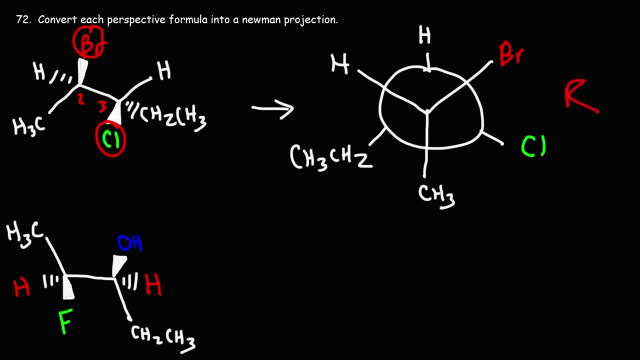 So that's how we can convert a perspective formula into a Newman projection. So remember, if it's on the wedge, it's going to be on the wedge. If it's on the wedge, put it on the right side. If it's on the dash, put it on the left side. 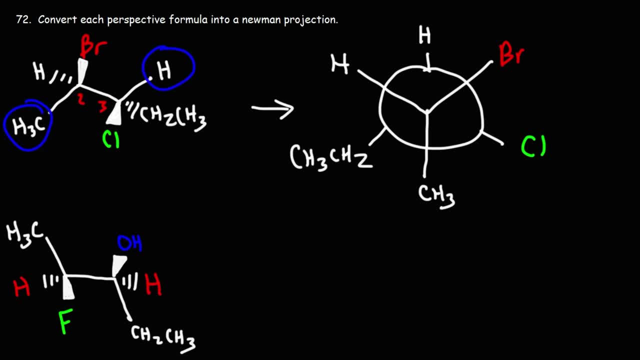 And then pay attention to these groups to see if they're anti to each other, if they're on the same side, to know if you have the staggered or eclipse conformation. Now let's focus on the next one. Here's carbon 2,, here's carbon 3.. 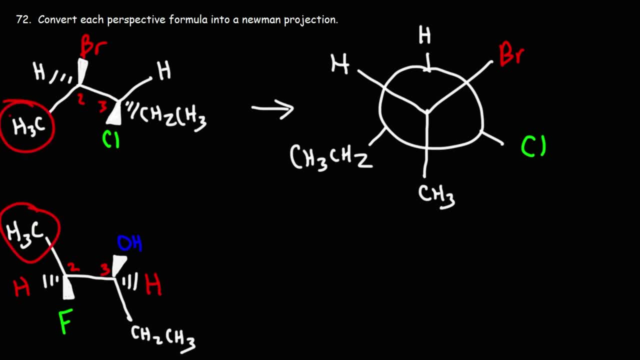 Notice that the methyl group is on top As opposed to being on the bottom. So we're going to draw the other version of the Newman projection. So the methyl group, instead of going down, it's going to go up. So here is that methyl group. 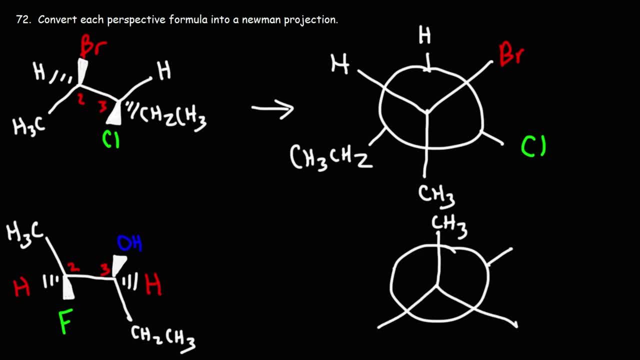 And here are the other parts of the structure. Now, the methyl group and the anti group. I mean the methyl group and the ethyl group are anti with each other. So if the methyl is going up, the ethyl group is going to be going down on carbon 3.. 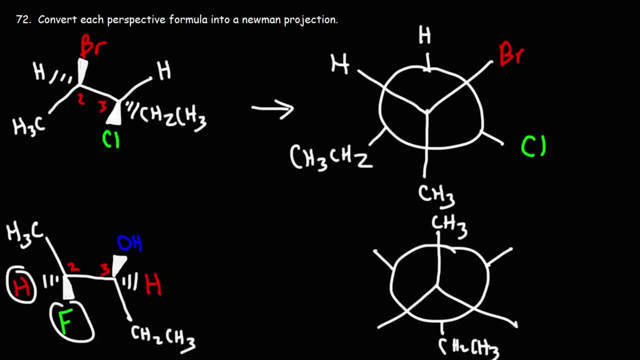 Now in carbon 2, we have a hydrogen and a fluorine. The hydrogen is on the dash, so we're going to put that on the left side. The fluorine is on the wedge. it's coming out of the page. We're going to put that on the right side.